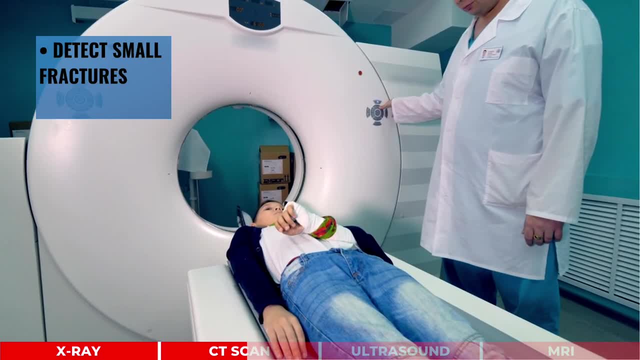 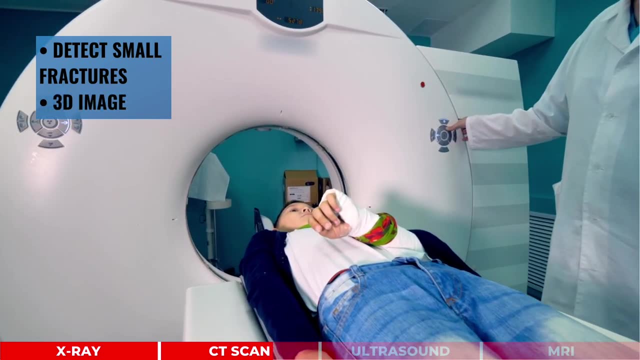 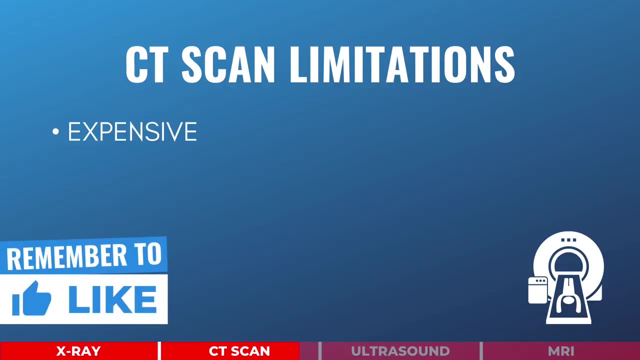 CT scan has many benefits. It can detect small fractures that may have been missed on the x-ray. It can also produce a three-dimensional image which makes it easier to locate the site of injury. CT scan has many limitations. It is relatively expensive and, compared to the 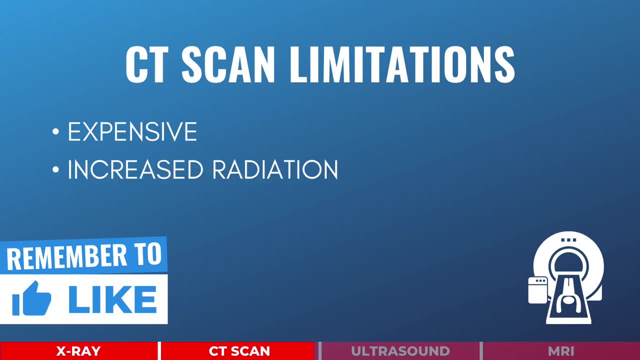 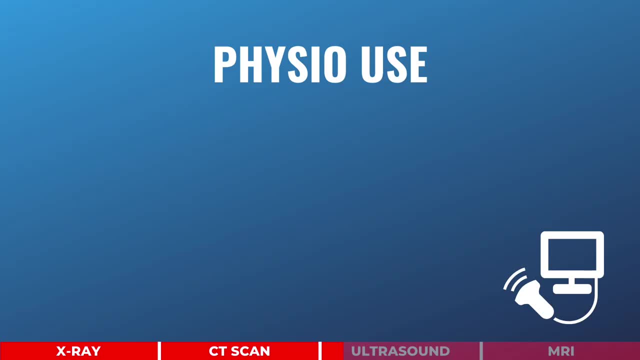 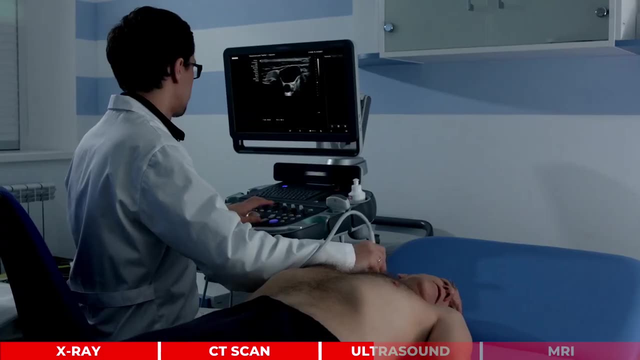 plain x-ray, it can expose a person to a greater amount of radiation. Ultrasound- Ultrasound uses high-frequency sound waves to produce an image. Physiotherapists commonly use ultrasound to evaluate soft tissues such as the muscle, tendon and ligament. 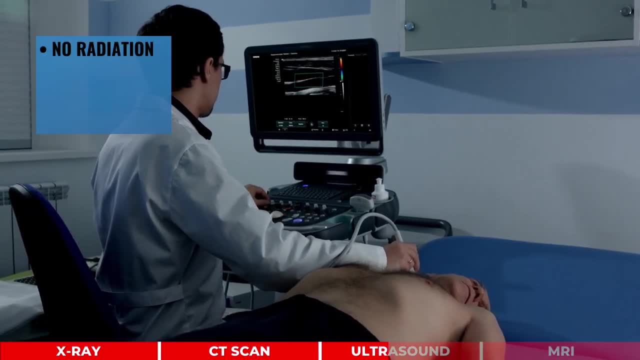 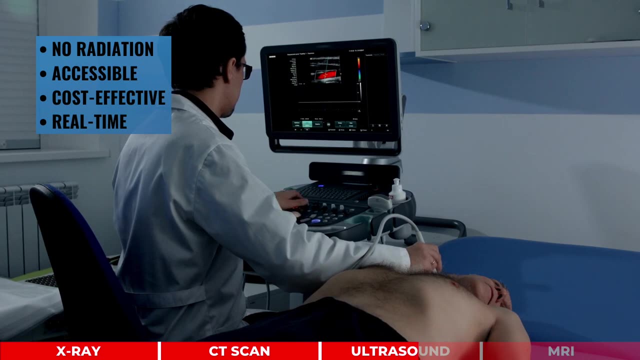 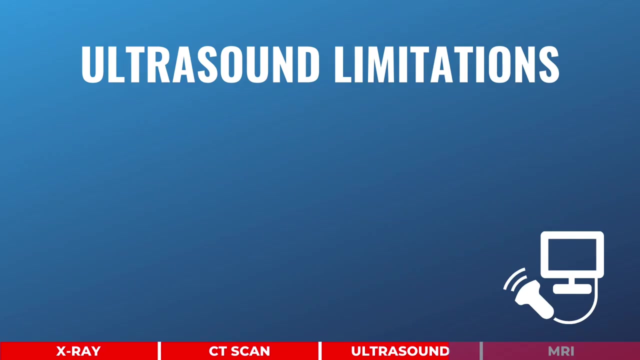 Ultrasound has many benefits: It does not expose a person to any radiation, They are readily available, cost-effective and, most importantly, they can be performed during movement. This is particularly helpful in the evaluation of shoulder impingement. The main limitation of ultrasound is it cannot penetrate the tissues and produce image of. 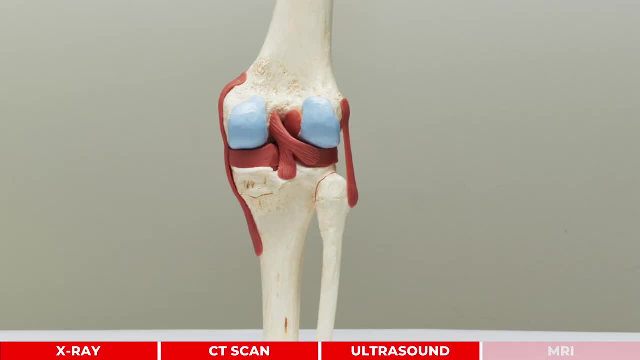 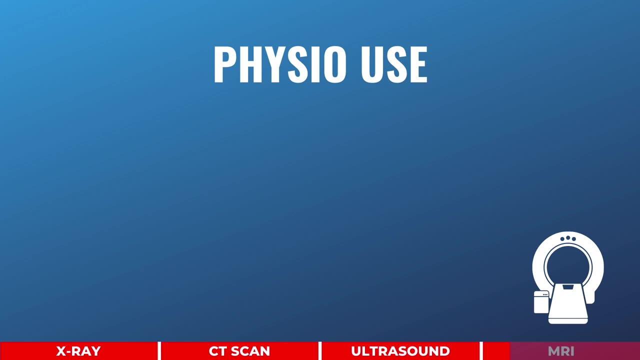 deep structures such as the meniscus and the ACL. MRI uses strong magnets and radio frequency waves to produce an image. Physiotherapists commonly use MRI to evaluate the meniscus labrum, spinal disc joint and soft tissues. 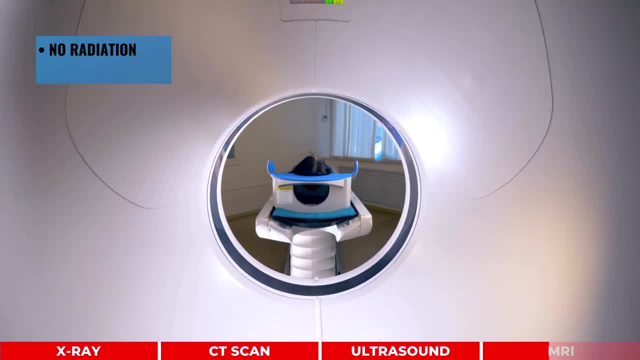 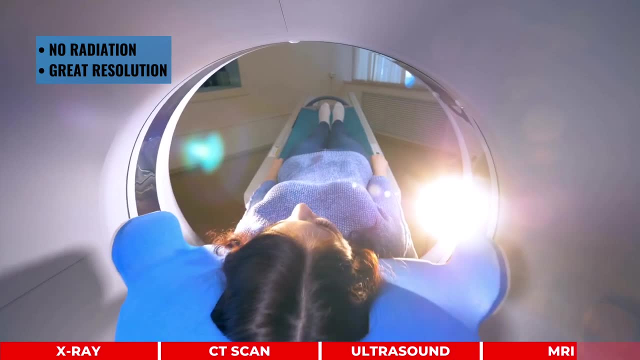 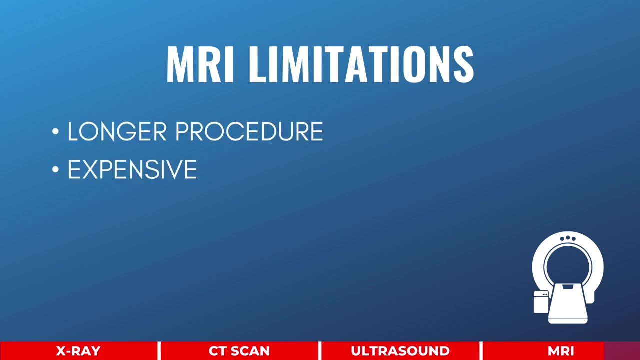 MRI has many benefits. It does not expose a person to any radiation. It provides detailed information about the body. This enables us to make accurate assessment of soft tissue injuries. MRI has many limitations: It takes a lot longer to perform, It is relatively expensive and it cannot be performed in people with certain metal implants. 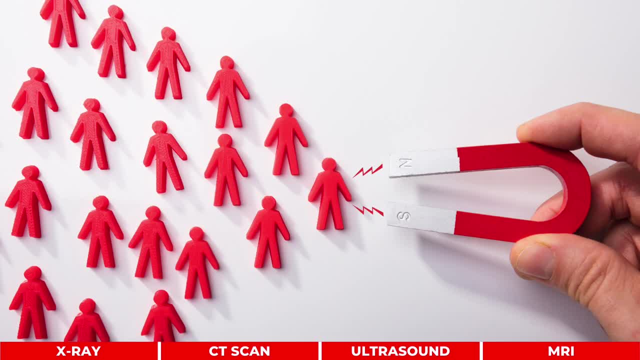 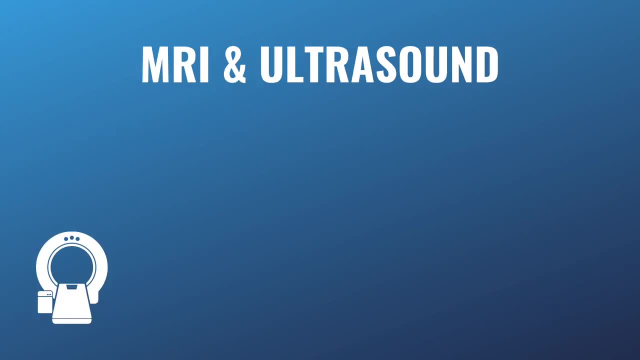 as some metals can heat up or attract to the magnet. In summary, X-ray and CT scan are often used to evaluate bony injuries such as a fracture. MRI and ultrasound are often used to evaluate soft tissue injuries. If you like the content from today's video, don't forget to subscribe. Thank you for watching. We will see you next time.